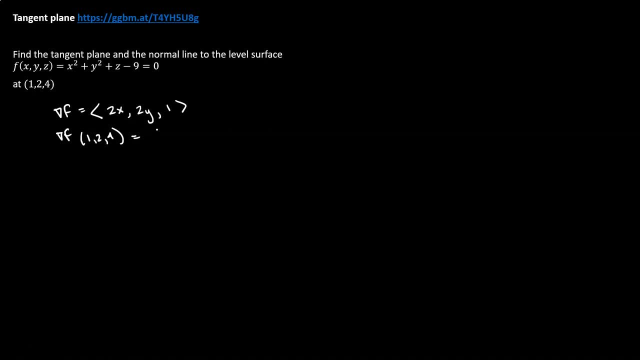 some point, like the one that's given to us, To find the vector 2,, 4, 1.. That's the vector that we would use for the equation of the tangent plane. Remember, the tangent plane needs a perpendicular vector, so our perpendicular 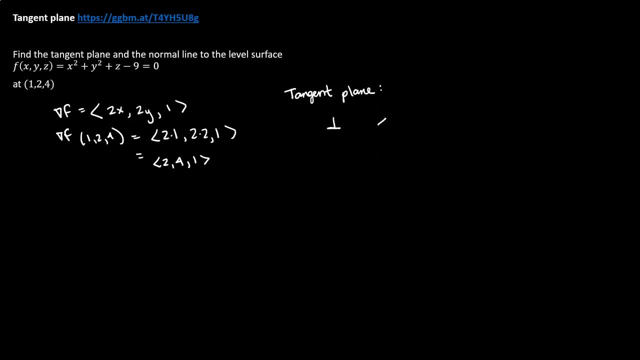 vector is the gradient vector. It also needs a point on the surface. We are given that point as 1, 2, 4.. So we can come up with the equation of the plane by taking each component and multiplying it by the change in the variable. 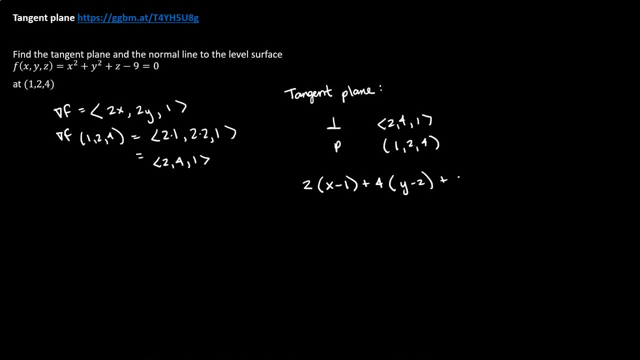 And then cleaning that up, And then cleaning that up, And then cleaning that up To get our final answer. To get our final answer for the tangent plane, For the normal line, we can write that using the parametric equations for a line where X is equal to the X value point. 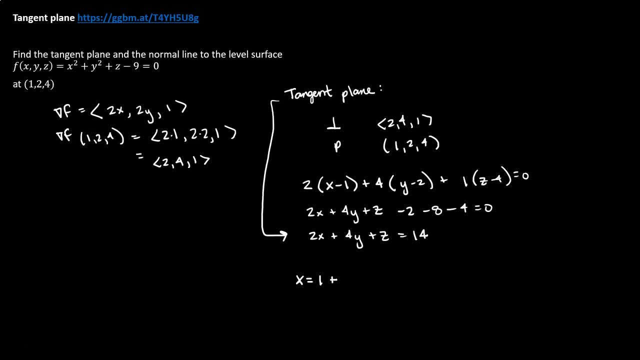 Where X is equal to the X value point plus the X component from our parallel vector times T, Y is equal to the Y value point plus the Y component from our parallel vector times T, and then Z is the Z coordinate plus the Z component times T. So this would be the normal line. 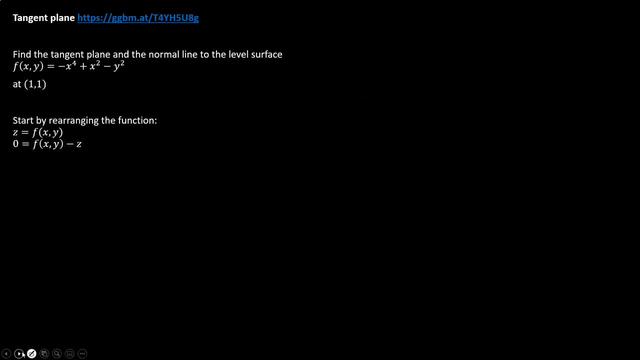 If we wanted to use this idea, using the gradient vector to find a tangent plane and a normal line for a function that's only of two variables, you might think: oh, same process, find the gradient vector, but notice that this gradient vector for 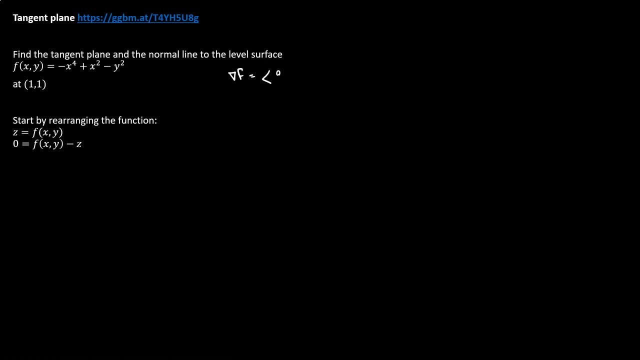 F. it's only going to have two components And our tangent plane needs a 3D vector as the normal vector. So what we can do is start by rearranging our function. Instead of having F of X, Y equals just an expression involving X and Y, we're going. 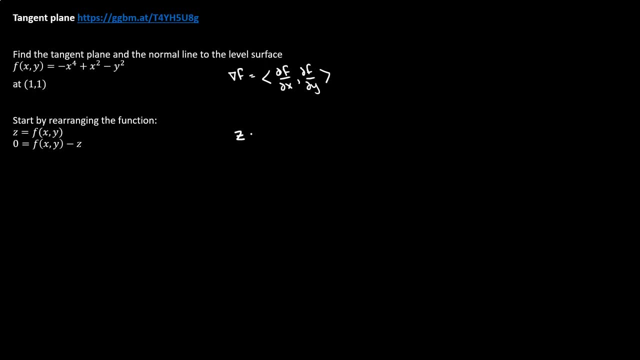 to rewrite our function, replacing F of X, Y with Z. And then we're going to create a new function. We're going to create kind of a dummy function where we subtract Z to the opposite side so that we have: zero is equal to negative, X to the fourth, plus X squared, minus Y squared. 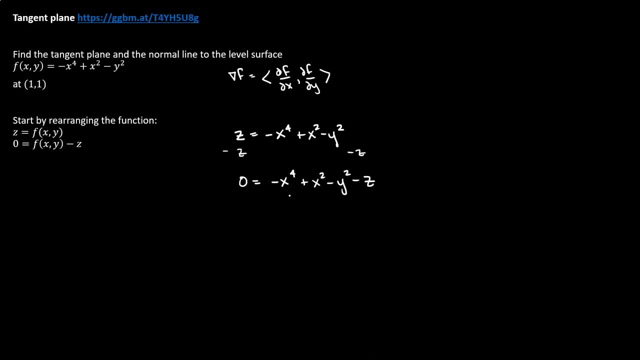 minus Z, And what we have on the right-hand side over here looks like a function of three variables. We can call that F capital, F function of three variables And then we can find the gradient vector of that and use that function to find the gradient. 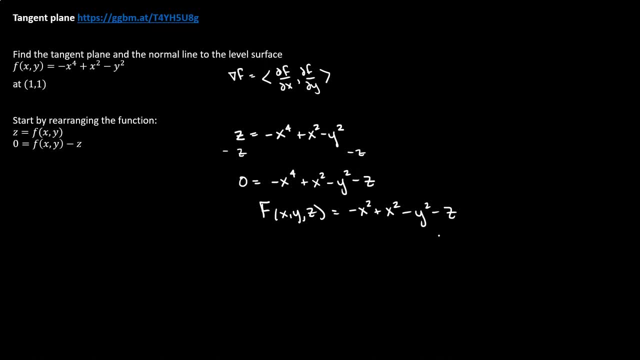 vector of that as our gradient vector in each of the formulas. So if we found the gradient vector of capital F, that would look like negative 2X. Oh, why do I have X squared written twice? Whoopsies, my X to the fourth turned into a negative X squared. 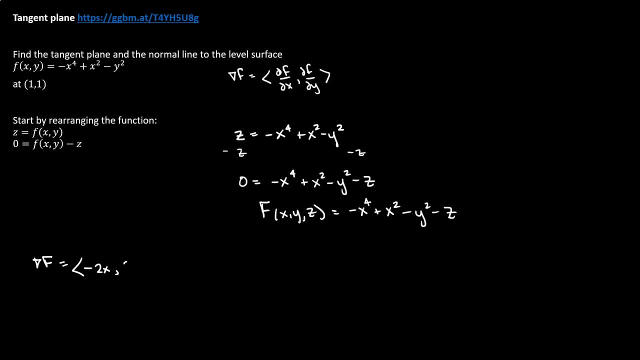 So we have negative X to the fourth plus X squared minus Y, squared minus Z. Let's calculate our gradient vector there. So we'll have negative 4X cubed plus 2X for the X partial, negative 2Y for the Y partial. 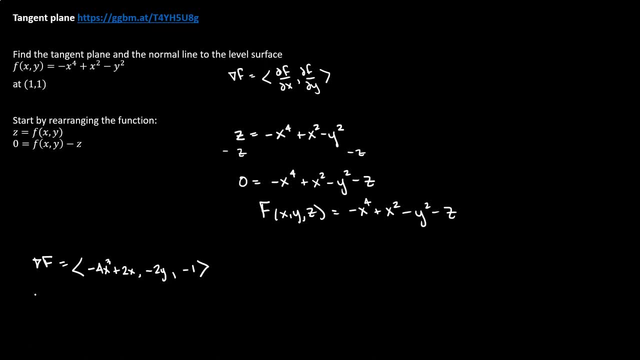 and negative 1 for the Z partial. If we evaluate our gradient vector for capital F at 1, 1, that's like X equals 1, Y equals 1. And in this case there isn't a Z to worry about. 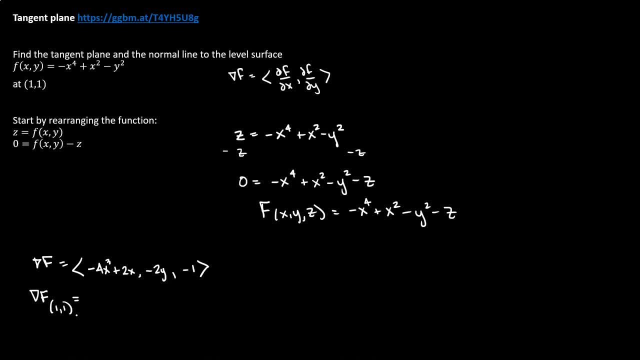 So we don't have to worry about what Z would be. However, if there were to be a Z, then you would have to calculate what Z is, But there's no Z to plug into, so we'll just plug in: X equals 1, Y equals 1..